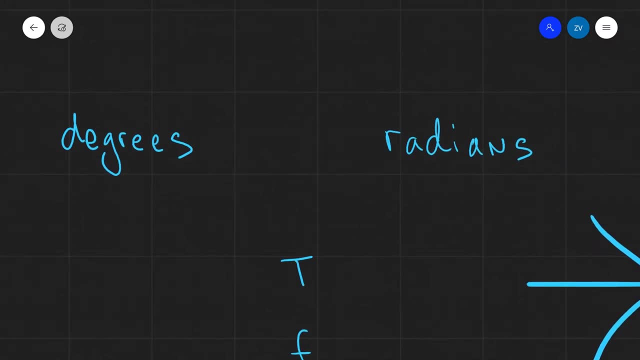 Now remember: if we wanted to convert from degrees to radians, what we need to do is multiply by pi and divide by 180 degrees. and if we're going the other way around, if we're going from radians to degrees, we need to multiply by 180 degrees and we need to divide by pi. A couple of useful ones: 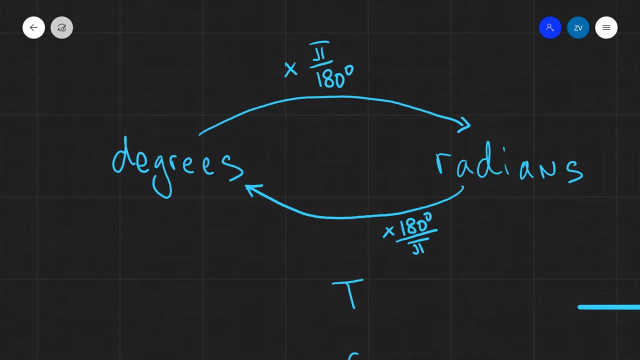 just to remember. so, one full oscillation, one full circle, is 360 degrees, which is equal to pi radians. additionally, 180 degrees is half of that, that's pi, and 90 degrees is half of that, that is pi over 2 radians. okay, next thing we need to remember are the time period, which is 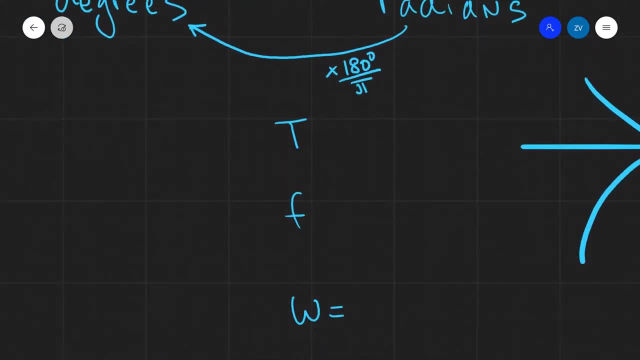 the time it takes to complete one full circle, essentially, the time it takes to complete one full orbit for an object which is moving in a circular motion. the time period is one over the frequency and the frequency is one over the time period. now, additionally, we can find the time. 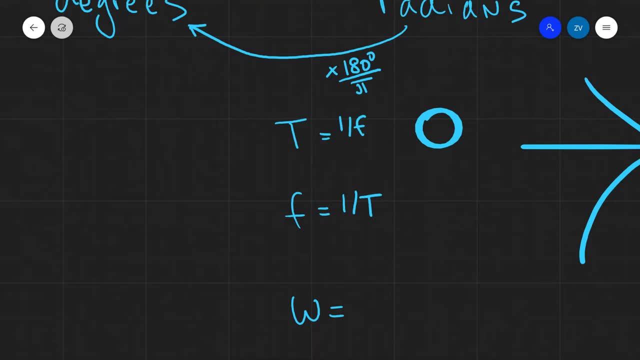 period or the velocity of an object that is moving in a circle, and let's say that the radius of this circle is r. now, if that's the case, the velocity is given by the circle and the radius of the circle is r, and the radius of the circle is r and the radius of the. 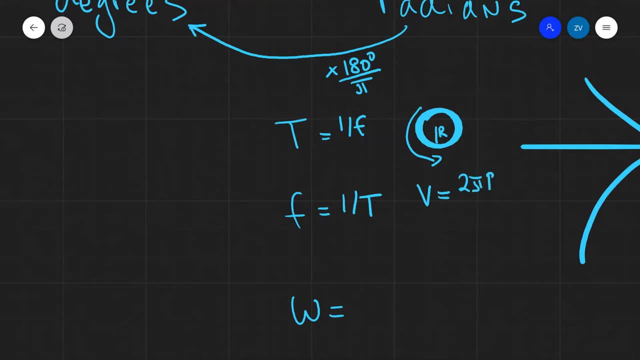 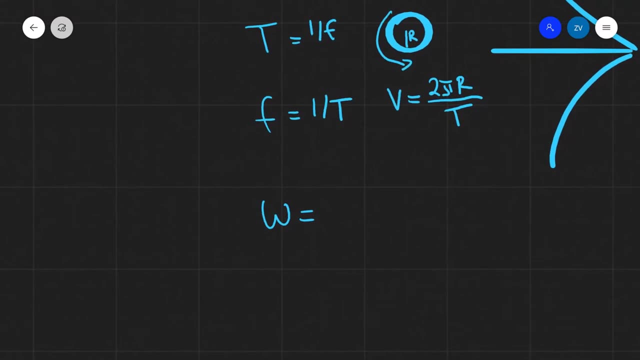 circumference, which is 2 pi r divided by the time period t. okay, next one, omega, our angular velocity. now, remember, our angular velocity tells us how many, uh, how, what angular displacement we are covering in a given time period. so it's the angular equivalent of normal linear velocity. 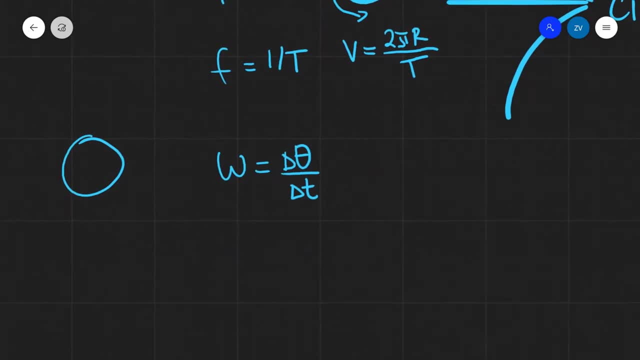 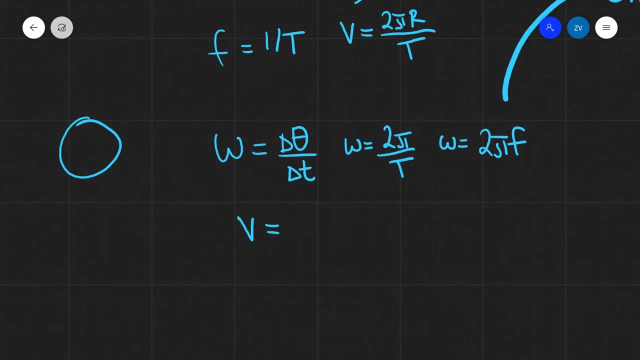 and the equations that we can use to find them are that omega is 2 pi over the time period, and because the time period is 1 over the frequency, we can also say that omega is equal to 2 pi f. additionally, the linear velocity and angular velocity are related by this equation. that v is equal to omega times r. 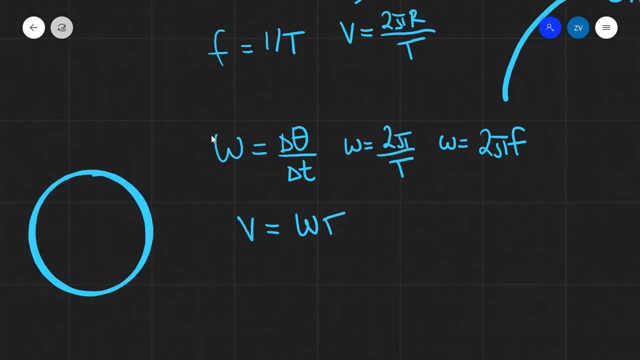 so, once again, the angular velocity, omega, that tells us how much angular displacement, let's say delta, theta, we cover in um, in in a second of rotation, whereas the linear velocity tells us the tangential velocity at a given point and what that magnitude is- they're related by v- is equal to omega r if we substitute one of those. 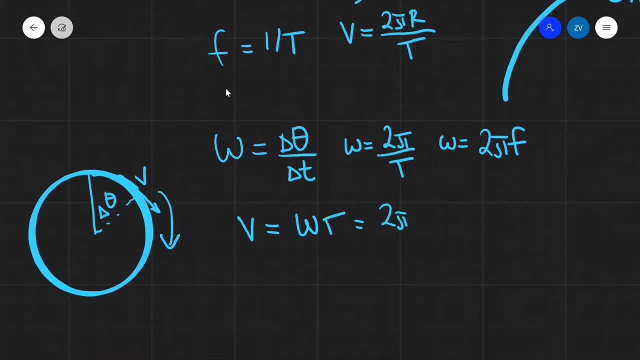 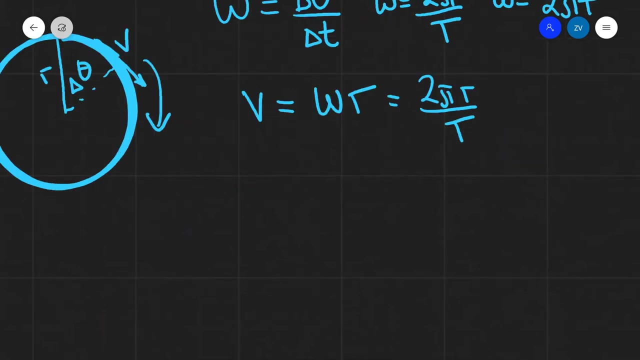 formulas for omega, for example, 2 pi r over t. if our circle is of radius r, we come back to our normal equation that the linear velocity is equal to the circumference divided by the time period. we will also need to remember how to convert from rpm, which is revolutions per minute. 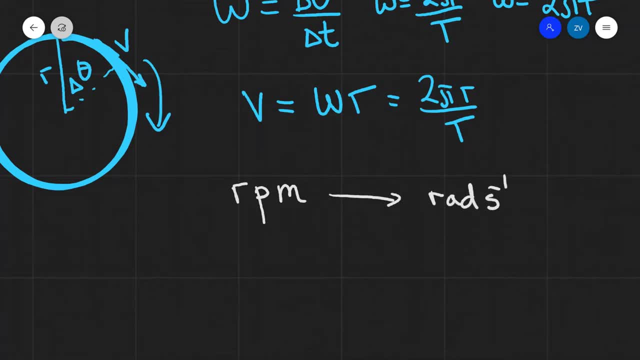 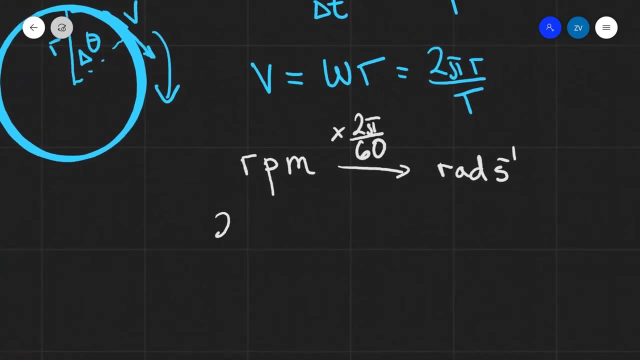 to radians per second. for our unit, for our angular velocity, the conversion factor, if we're going from rpm to radians per second, is multiplying by 2 pi and then divided by 60.. for instance, if i had something which was spinning at 200 revolutions per minute, so rpm, so that means that it does 200. 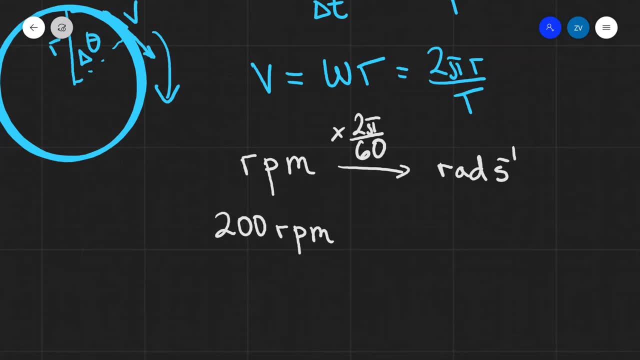 complete cycles in one minute. so the actual distance, the actual angular displacement that, uh, that it's going to cover, is going to be 200 full circles, which is 200 times 2 pi, and the amount of seconds in one minute is 60. so because it's per minute, we per 60 seconds and if we put 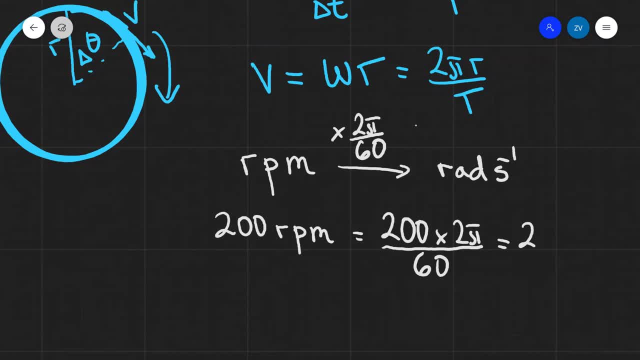 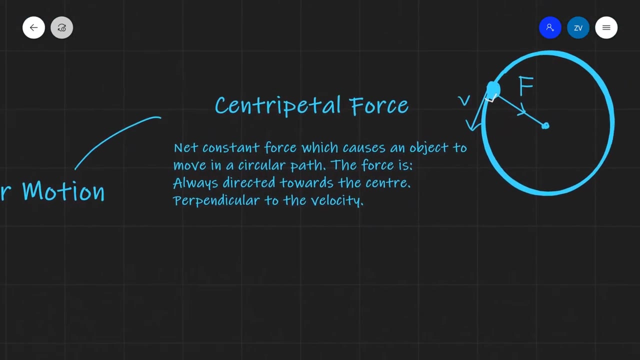 that into a calculator, we get about 20.9. call that 21 radians per second. okay, so let's have a look at centripetal forces next. now, what is a centripetal force? so that's a net force which causes the object to move in a circular path, and that force has two really. 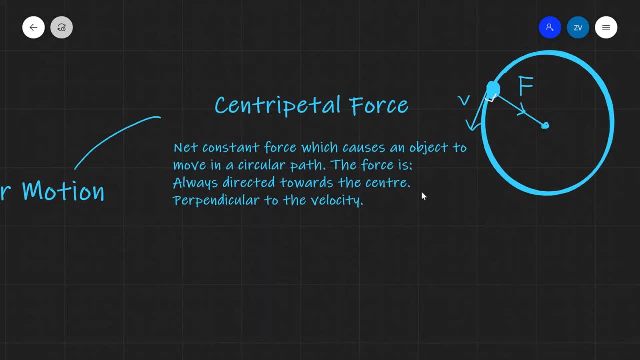 really important features. number one, it is always, always directed towards the center. and number two, it is perpendicular to the linear velocity of that object. so that's why it's called the centripetal force, if you're looking at something like a нейmonic, which is a very common object. a common examples of those forces are, for example, the: 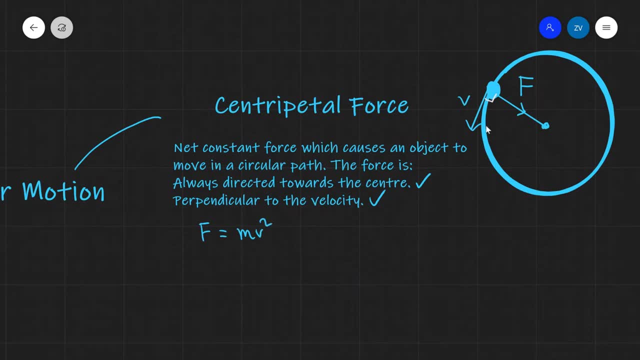 tension. if you have something which is being rotated in a circle, it could also be the gravitational force, it could be the frictional force, etc. the formula for it is given by, which is towards the center of rotation, and that centripetal acceleration is given by the formula. 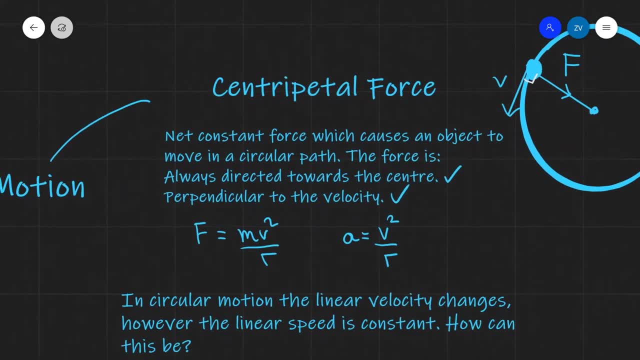 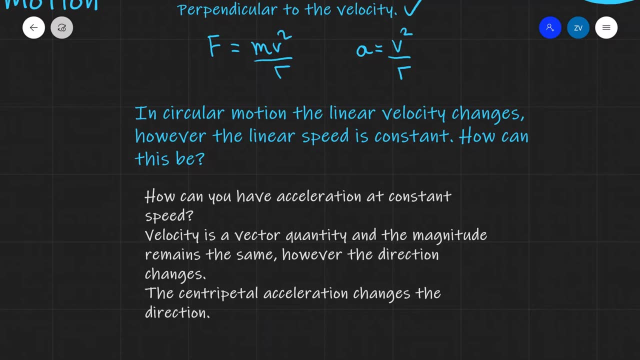 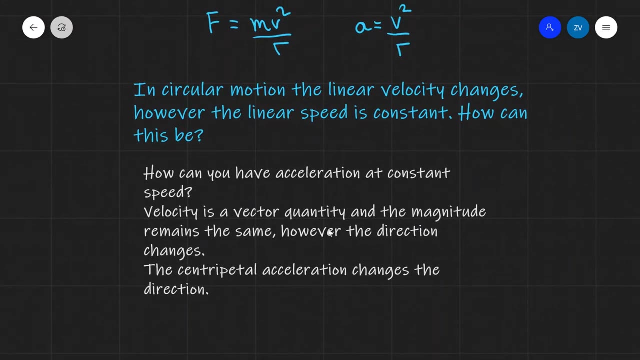 of v squared divided by r, a next one now, in circular motion, the linear velocity changes. however, the linear speed is constant. how can this be remember? you can have acceleration at constant speed because velocity is a vector quantity and only the magnitude, ie the speed remains the same. however, the direction is constantly changing, so the centripetal acceleration. 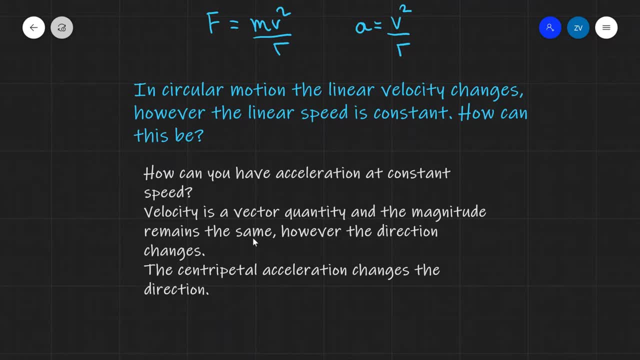 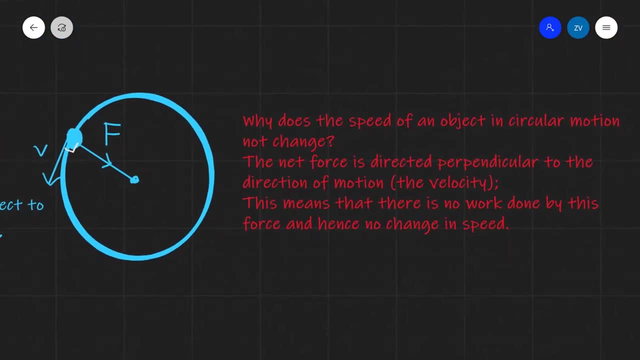 changes the direction of motion only now. this next question is really, really, really important. that's why i've put this in red. why does the speed of an object in circular motion not change now? the reason for that is because the net force is directed perpendicular to the direction of. 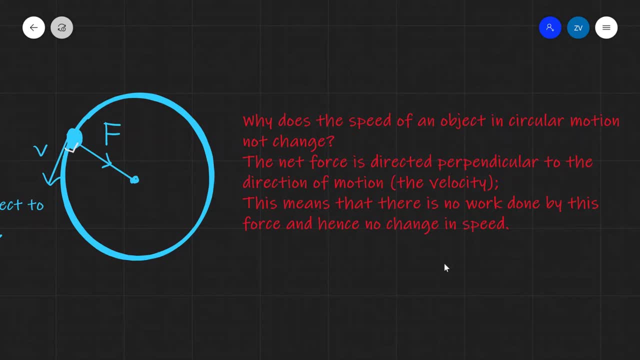 motion, ie the velocity. now this means that there is no work done by this force to change the speed of an object in circular motion. so the net force is directed and hence there is no change in the speed. remember, work done in general is equal to the force times. 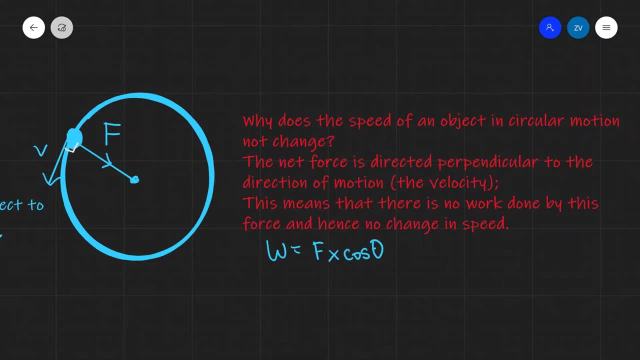 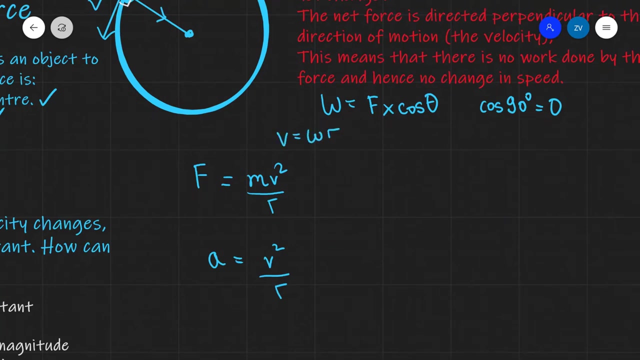 the displacement times. the angle between them- so it's fx, cos, theta and cos of 90 degrees, is equal to zero, which means that the work done will be zero if the force f and the displacement x are perpendicular to each other. now, because v is equal to omega r, we can rewrite the following two equations: one for the centripetal force and 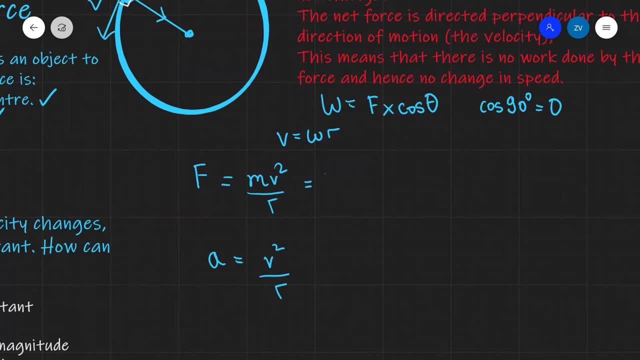 one for the acceleration, as the following f is going to equal m omega r squared divided by r, which is going to give us m omega squared r squared divided by r. we can cancel those out, which is going to give us m omega squared times r. similarly for the acceleration. 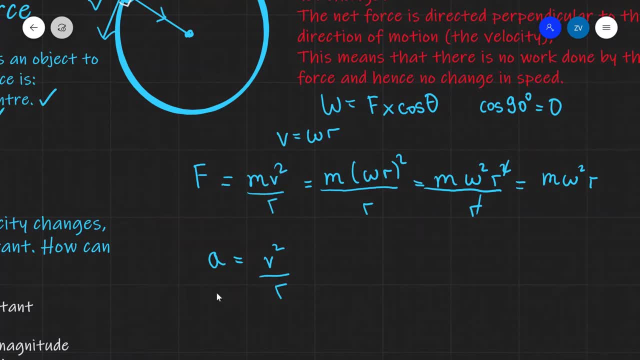 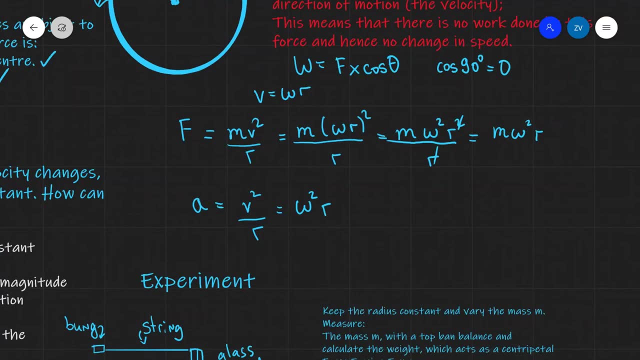 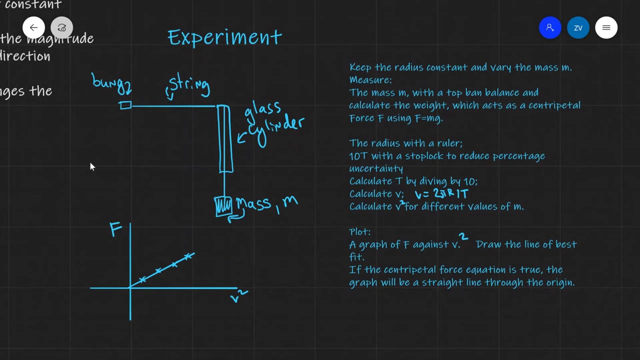 this is exactly the same equation, just without the mass in front of it. this is going to equal to omega squared times r. let's have a look at an experiment to try and investigate circular motion. so we have the following setup over here in which we have a. 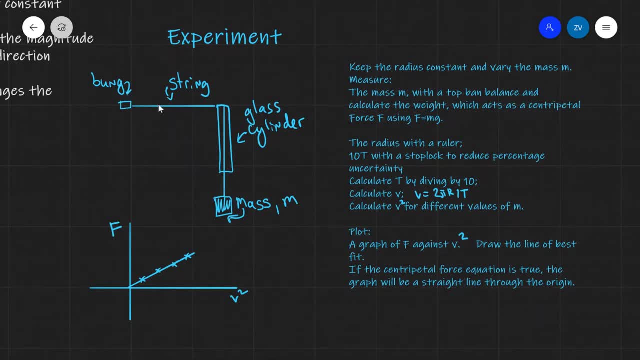 bunk which we're going to spin, that's connected on a piece of string that goes through a glass cylinder and it reaches a mass on the other end. i'm going to try and keep the radius of the mass constant. we would normally try and do that with a, with a marker we could have that we have placed. 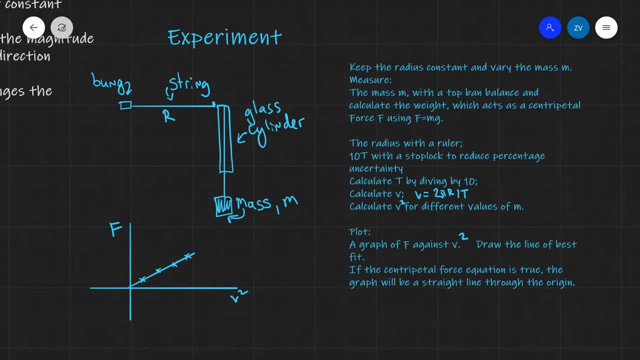 on this end of the string, just where it meets the glass cylinder, and we're going to be varying the mass m. there are many different variations of this experiment, so something could come up in a question which, for example, you are keeping the mass constant but you're varying the. 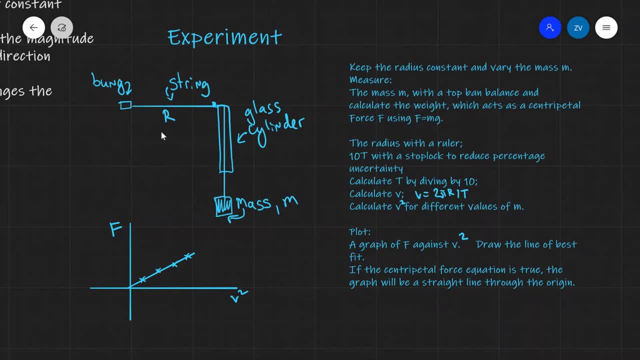 radius r. so be prepared, be prepared to be quite flexible in how we're going to approach this problem. we can measure the mass m with a top-hand balance and then we could calculate the weight which actually provides the centripetal force, and that weight is providing the centripetal force once. 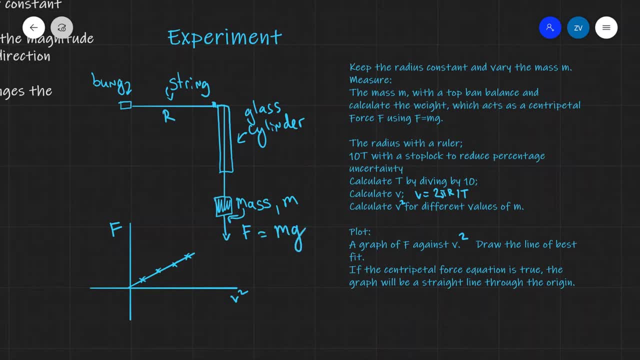 again, which is equal to just mg. we're going to measure the radius r with a ruler and then we're going to be timing 10, at least 10, i would say: 4 oscillations, 10 full time periods with a stop clock, and we're doing. 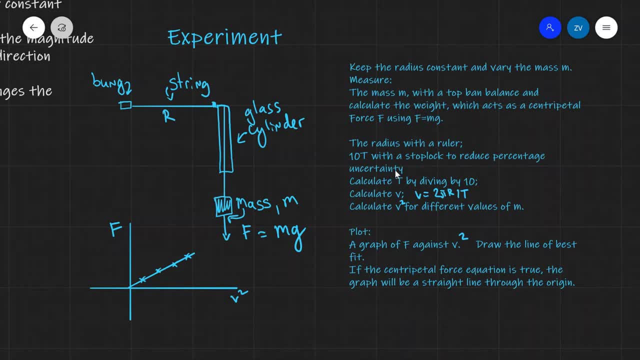 that to reduce the percentage uncertainty, improve the accuracy. in our experiment we're going to calculate t by dividing by 10. after that we could calculate our velocity using v is equal to 2 pi r over t, and then we could calculate v squared for different values of m. in terms of our analysis, 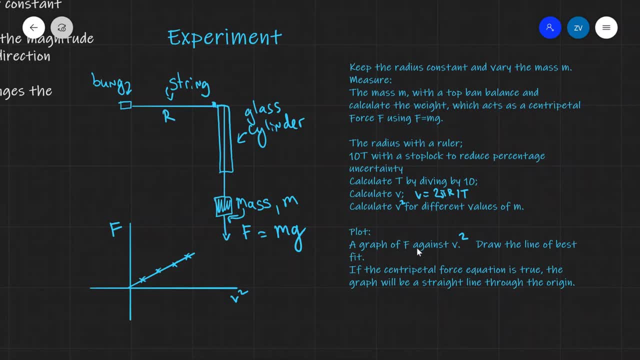 we're going to plot a graph of the force which is just m, and then we're going to plot a graph of the force which is just mg against v squared. now, if the um, if the formula for centripetal force is true, the graph will be a straight line through the origin. additionally, we could use this graph to 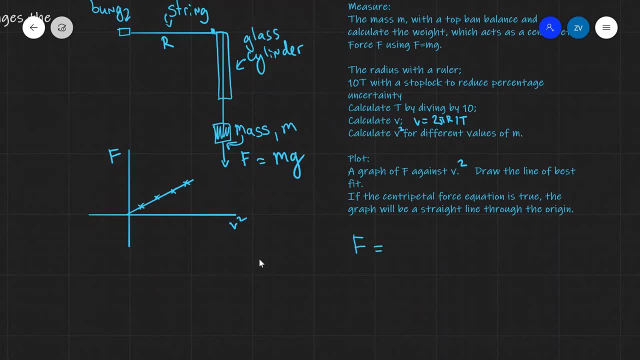 determine the mass of the bunk, should we wish to remember that f is equal to mv squared divided by r? now, if we have f on the y-axis, we have v squared on the y-axis, and if we have f on the y-axis, we have v squared on the x-axis. what's left for our gradient and our intercept is zero. so let's just. 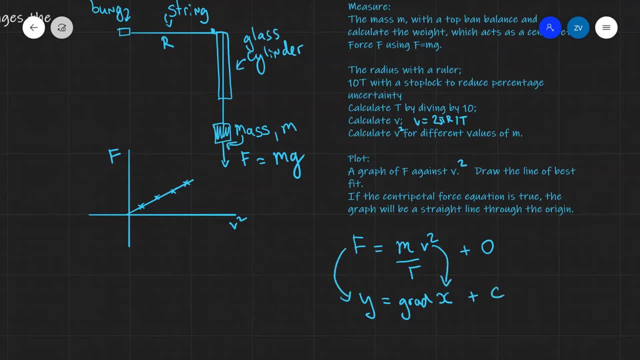 write that over here. so f is on the y-axis, v, squared, is on the x-axis, c is zero. our gradient is the mass of the bunk divided by the radius. so we could say that our gradient- let's call that grad- is equal to m over r and depending what is known in this question, for instance if we know, 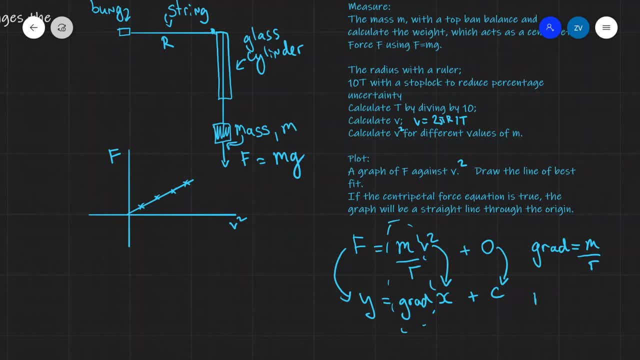 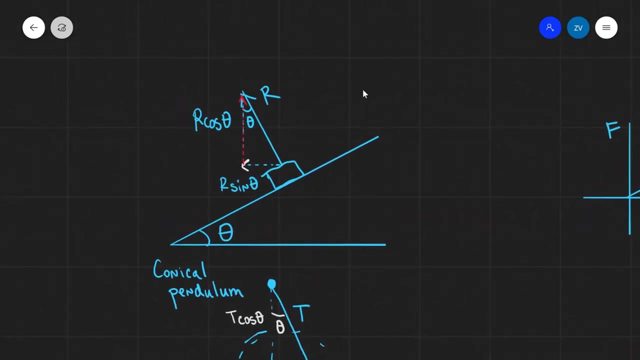 the radius and we wanted to find out the mass of the bunk. we could say that the mass of the bunk will be equal to our gradient. it's called grad times r okay, now let's have a look at circular motion at an angle. so we have something like a car which is turning to the left- the normal. 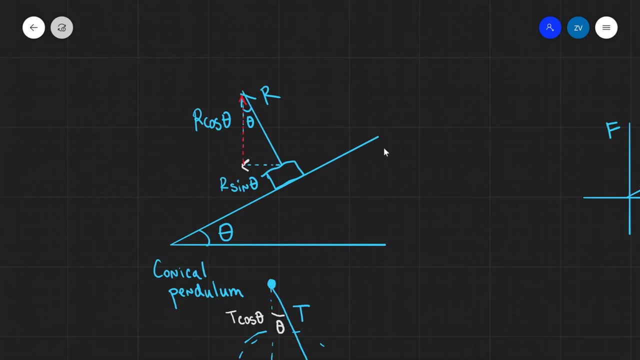 reaction r is always at 90 degrees to the uh to direct to the angle of the slope, so that means that this angle here is going to be equal to this angle here. this is because of similar triangles, by the way, and we can split the normal reaction r into two components: r, cos, theta and r. 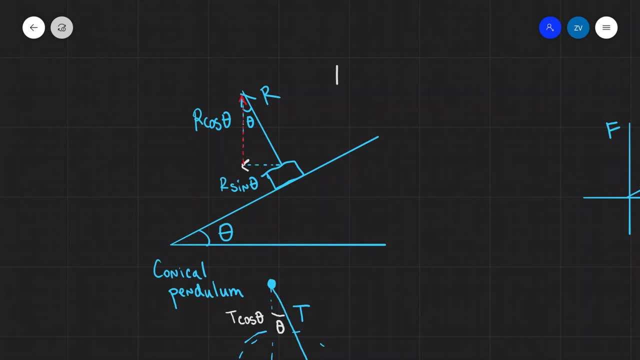 sine theta. now, in this setup, r cos theta is going to be balancing out the weight, because that's the vertical component acting upwards. so if the car is not moving up or down, this that better be equal to the weight. mg and r sine theta. this component of the normal reaction will actually be providing. 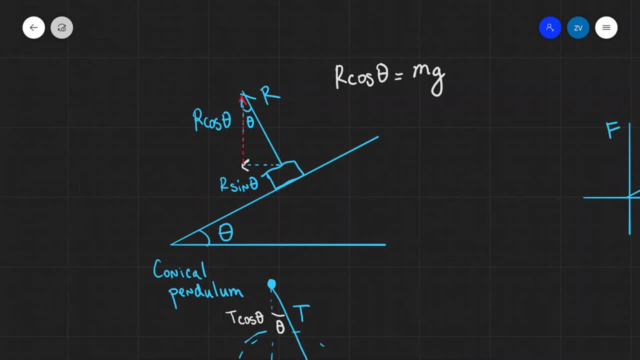 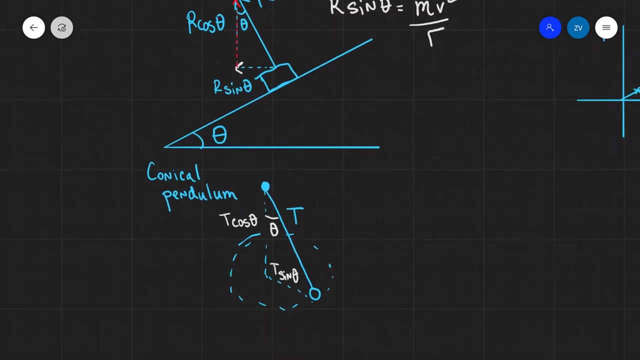 the central reaction. so we can split the normal reaction r cos theta and r sine theta and r cos theta because that's the net force acting towards the direction of turning. so r sine theta is going to equal to mv squared divided by r. very, very similar in a conical pendulum, that is, at an angle theta. 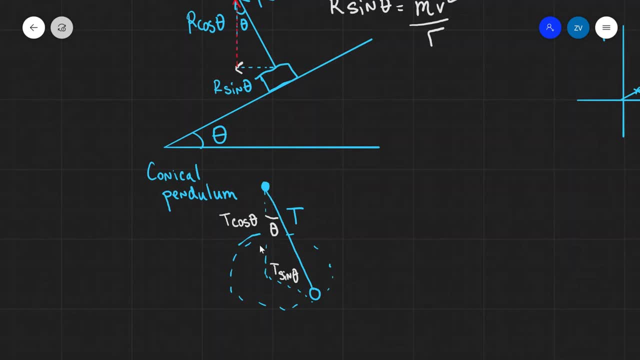 the vertical component is equal, is the adjacent, which is equal to t cos theta, and that is equal to mg. additionally, we can also do the same thing with the vertical component, which is equal to mv squared divided by r, which is equal to the set of four of the direct forces over. 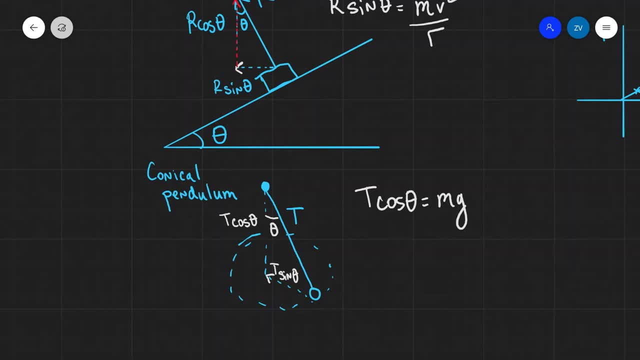 here and the horizontal component thelando at the court. that goes using the notation force. but as you can see today, suddenly the horizontal component is the one component which is acting towards the center of rotation. that actually provides the centripetal force. so t sine theta is equal to mV squared over r- circular motion, an angle could be represented. 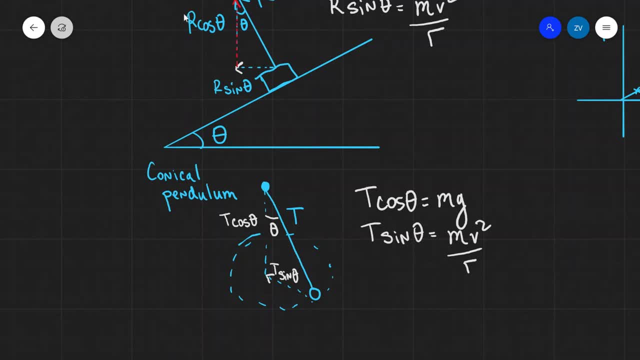 in many different situations. for instance, you may have the lift force or some frictional forces which is making something and turn. so please be aware, to ensure tension and the normalвонterminally, the non-tenant volts are maintain the interval between the hits. Khalid, and I refer to theige of handed expressions as external forceável. 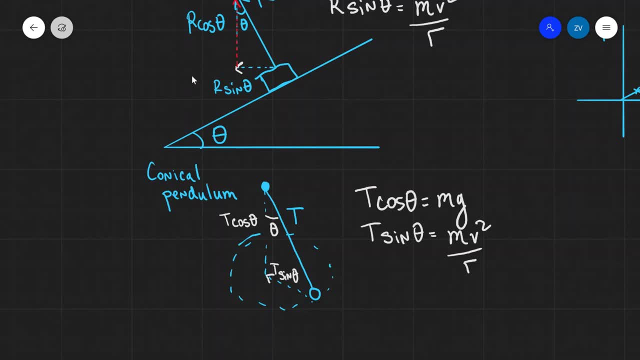 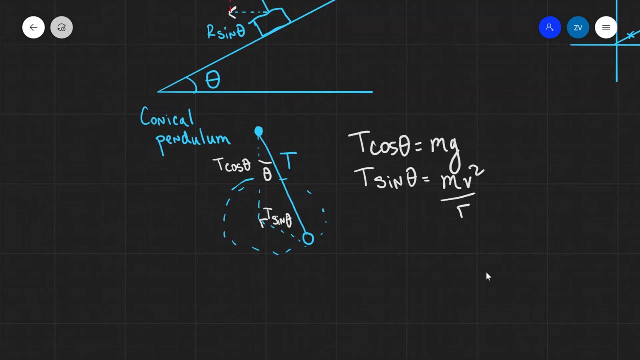 reaction are not the only examples of forces in which this type of problem could be applied to. A typical problem would ask us to calculate the speed in this situation. If that's the case, we need to have a look at this system of two equations. The way we would normally do it is just rearrange one of the. 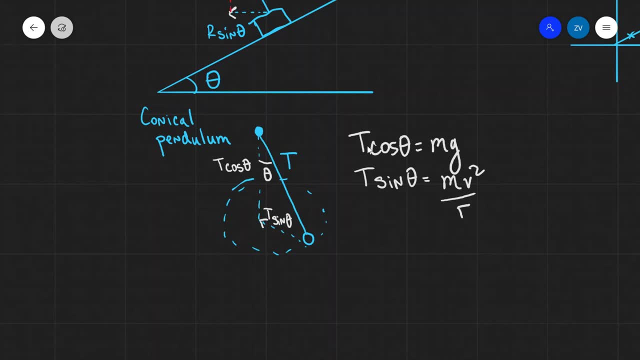 equations for one of the unknowns, for instance T, We can say that T is going to equal to Mg over cos theta, and then what I'm going to do is I'm going to input this equation into this expression over here. so, rather than T, sine theta, 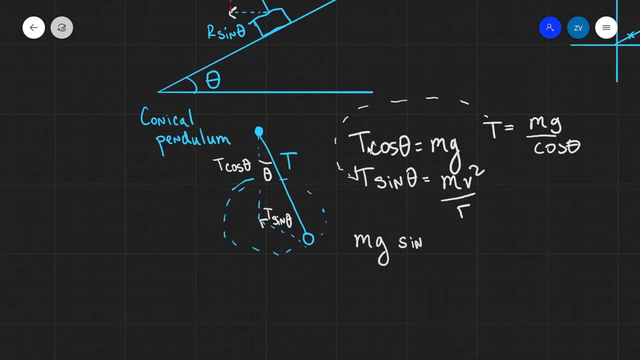 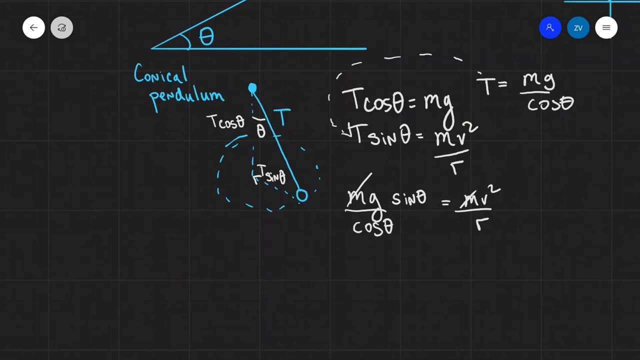 I'm going to write Mg sine theta over cos. theta is equal to Mv squared divided by R. Notice that Mv squared is equal to Mv squared divided by R. Visualization is vertical and vertical, So the equation is vertical and vertical. my other unknown, which is the mass in this case, is going to cancel out and sine of a cos is equal to. 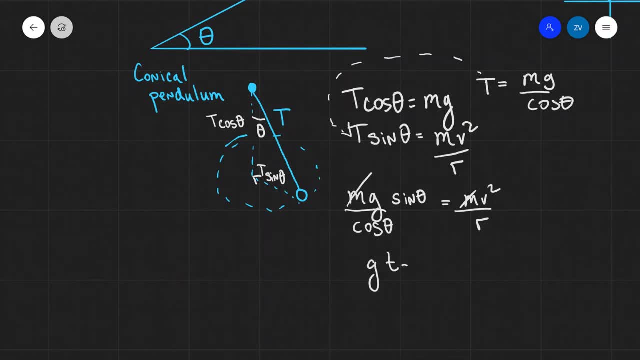 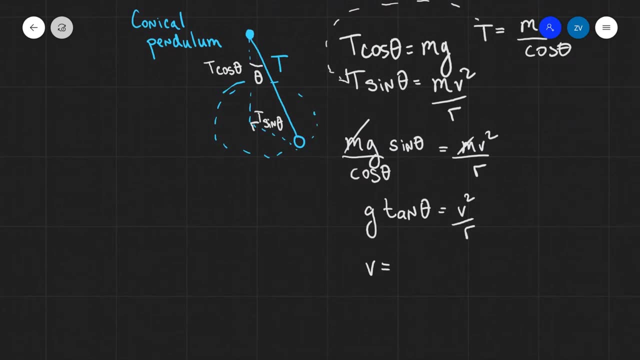 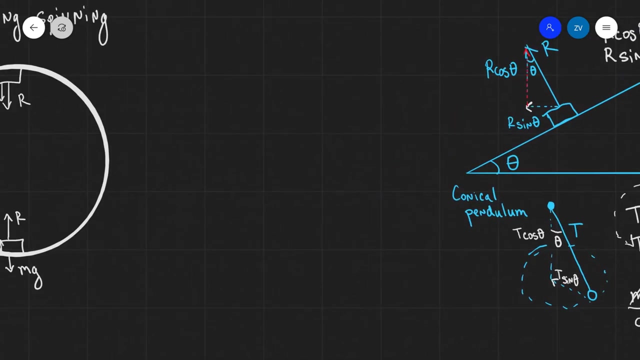 tan. so i'm going to get that g tan of the angle is equal to v squared divided by r. in other words, v is going to equal to the square root of gr tan theta. okay, and finally, let's have a look at vertical circular motion. so this is just an example of 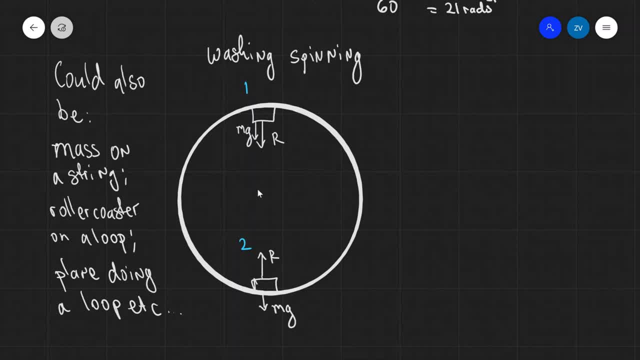 some washing which is spinning in the drum of a washing machine, but this could be a bunch of other situations as well. for example, it could be a mass on a string that is being moved in a vertical circle, or it could be a roller coaster loop on a plane. 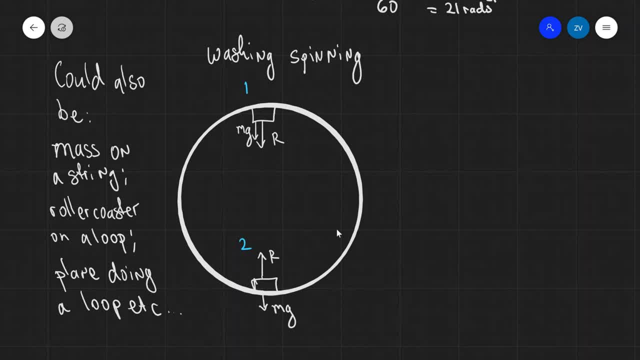 doing a vertical loop, etc. so, etc. Now let's imagine two positions, 1 and 2.. Now notice that in position 1, Mg and the normal reaction R are in the same direction. Position 2, Mg and R are in the opposite directions. Let's 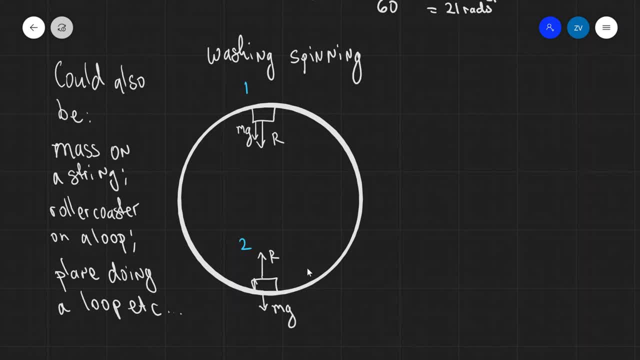 apply Newton's second law for each of those directions, each of those positions. So for position 1,, Ma is going to equal the sum of the two forces. Now they're in the same direction, so I'm going to add them, So I'm going to say this is equal to Mg plus R. Now remember my 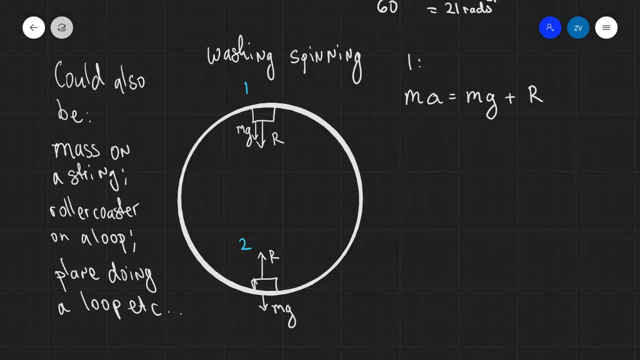 acceleration- in this case, because we're moving in a circle now- is centripetal. So this is going to equal to Mv squared over. R is going to equal to Mg plus R. Now this means that in position 1,, 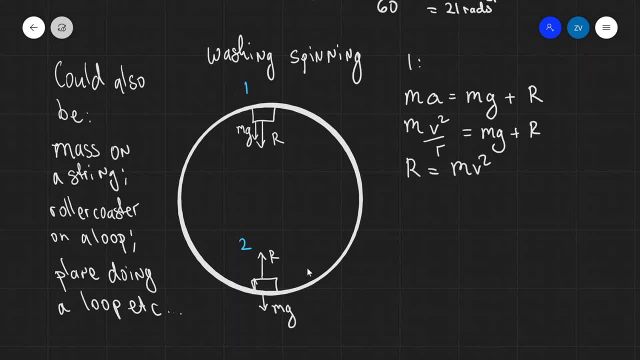 the normal contact force will be equal to Mv squared over R minus Mg. Now in position 2, we're going to follow exactly the same procedure. We're going to write that Mv squared over R is going to equal to. now we're going to have to. 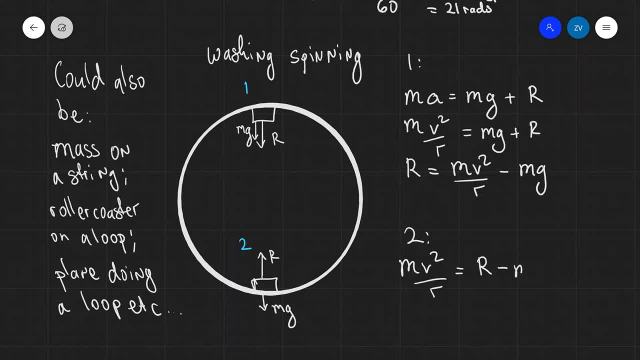 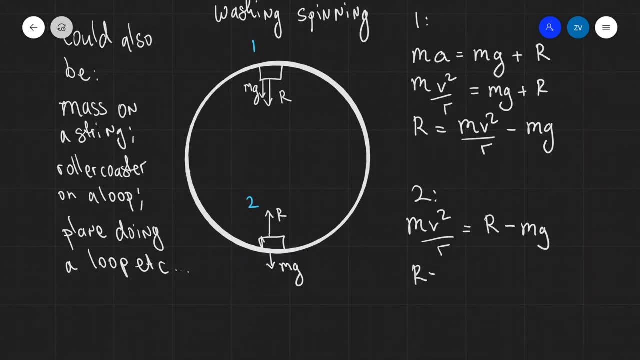 take them away and it will be R minus Mg, because we can see that they are in the opposite direction. So just rearranging it for R once again, we're going to get that R will be equal to Mv squared over R plus Mg. Now notice that R will be the greatest in position 2, because we